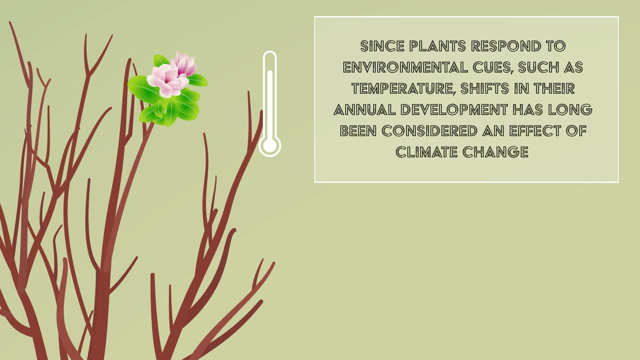 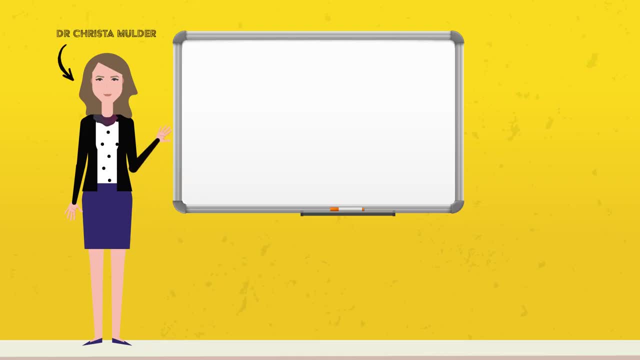 shifts in their annual development has long been considered an effect of climate change. However, significant warming does not always lead to earlier flowering. Dr Krista Mulder from the University of Alaska, Fairbanks, recognized that plant flowering may not be directly related with 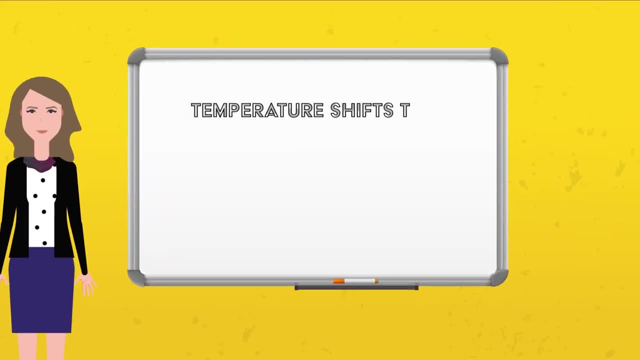 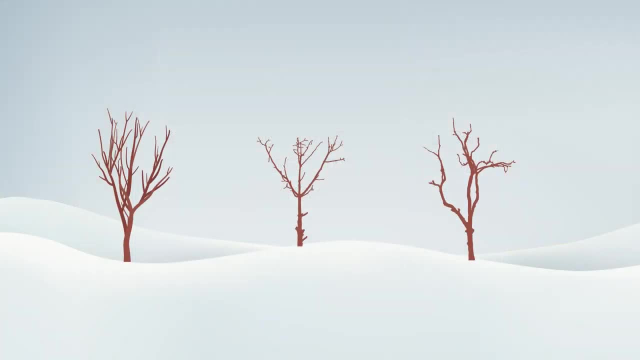 spring temperature. Rather, she hypothesized that temperature shifts that occurred in previous years may influence the effects of rising temperatures in the flowering year. Dr Mulder and her colleagues began by analyzing subarctic plant communities in Canada: An analysis of decades of data for 39. 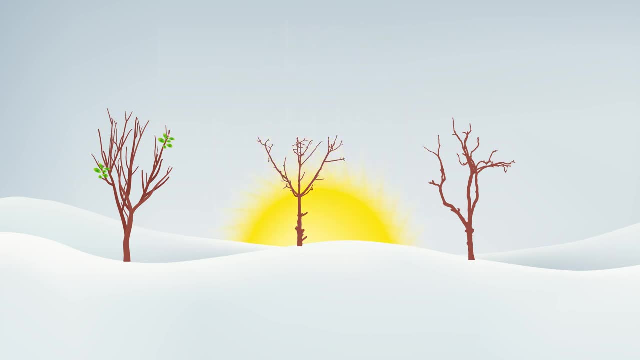 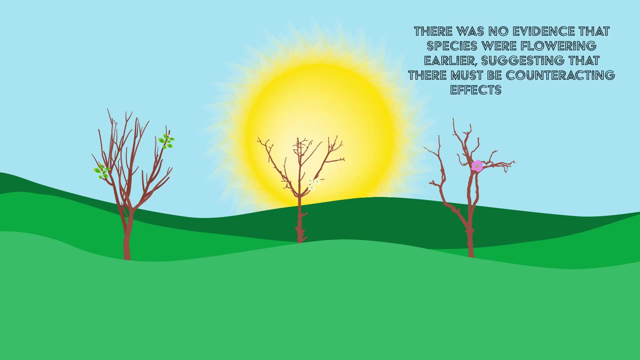 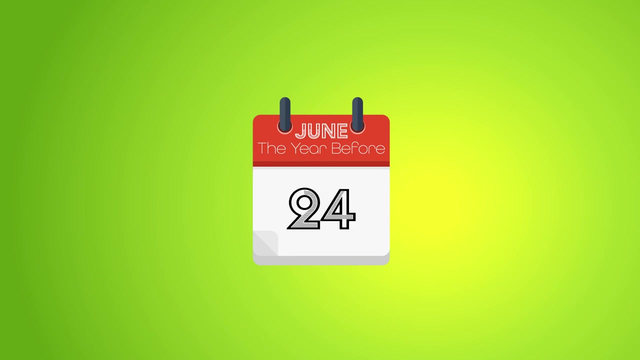 plant species yielded surprising results. Despite significant warming over time, there was no evidence that species were flowering earlier, suggesting that there must be counteracting effects on rising temperatures. Diving deeper, the scientists focused on the early summer temperature in the year before flowering, a time when the buds start to develop Their results. 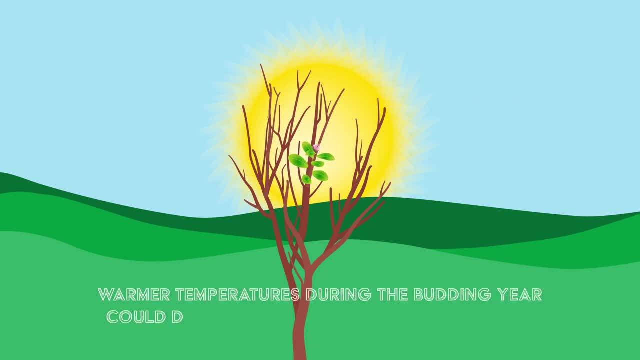 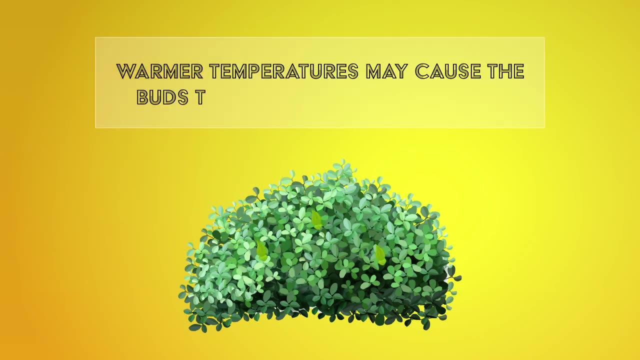 suggested that warmer temperatures during the budding year could delay flowering time in the next year. Though the causes are still uncertain, the team hypothesized that warmer temperatures may induce early dormancy. Next, Dr Mulder focused on understanding the development of the bud. 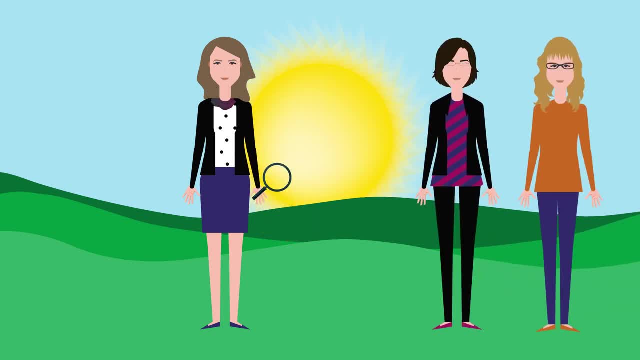 itself. In a collaboration with Dr Pamela Diggle and Eileen Schaub, she investigated how variation in temperature affected the flower development of the shrub lingonberry, also known as lowbush cranberry. The researchers headed into the field to collect flowering shoots at different stages. 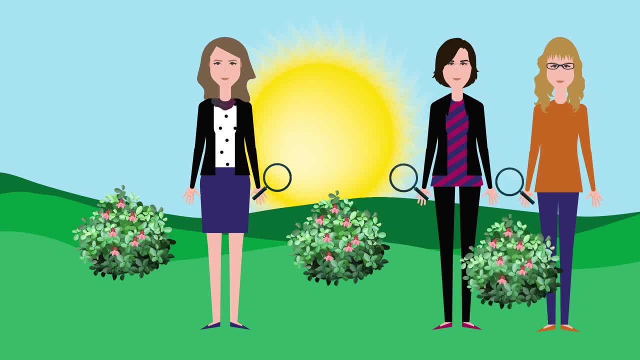 of development from warm and cold sites in the boreal forest and conducted an anatomical assessment of the buds. In sites where it was warm in spring and the ground thawed, the shrub lingonberry was the first to develop flowering shoots. 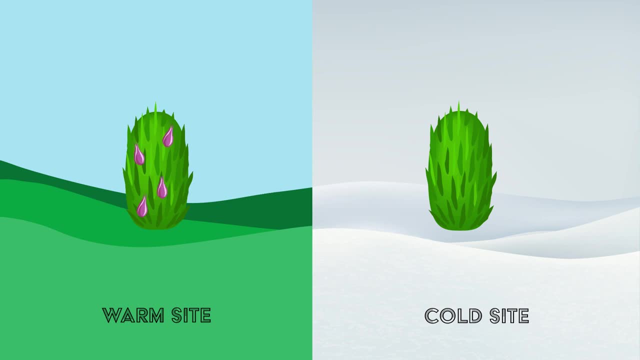 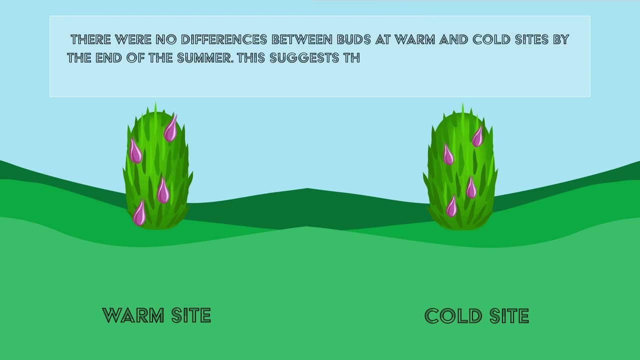 In sites where it thawed early, buds started to develop early. However, because the buds all stopped developing at the same stage, there were no differences between buds at warm and cold sites by the end of the summer. This suggests that at a certain point, flower development is controlled. 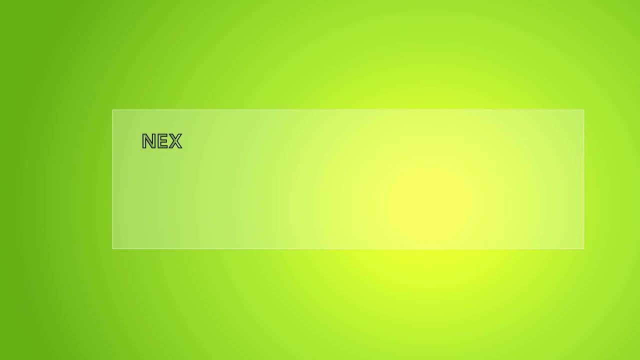 by internal processes within the plant. Next, Dr Mulder and her colleagues looked at what happened in six plant species when temperatures are higher than normal. They created artificial open-top chambers to warm the plots and split them into four treatments. Plots warmed in the. 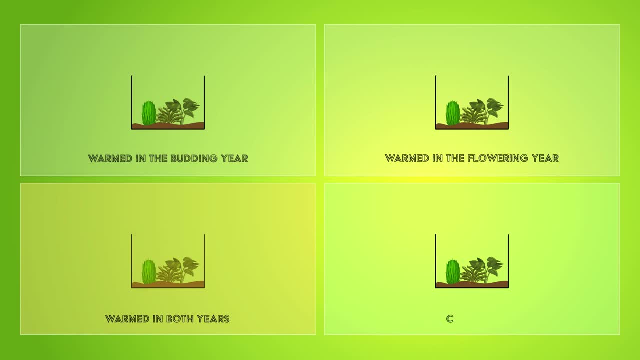 budding year: Plots warmed in the summer. Plots warmed in the fall. Plots warmed in the fall. Plots warmed in the flowering year. Plots warmed in both years and a control group For most species. plants that had been warmed only in the flowering year flowered earlier.